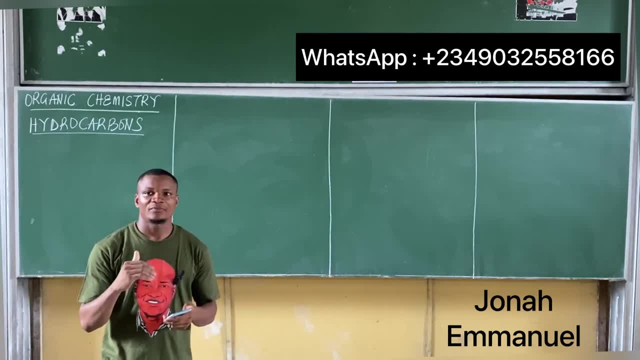 Take a paragraph. take a paragraph On the basis of structure, on the basis of structure comma. on the basis of structure comma, hydrocarbons are divided into. hydrocarbons are divided into two main classes. On the basis of structure, hydrocarbons are classified into two main. 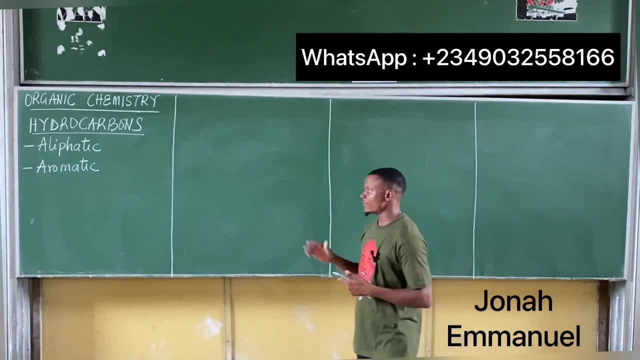 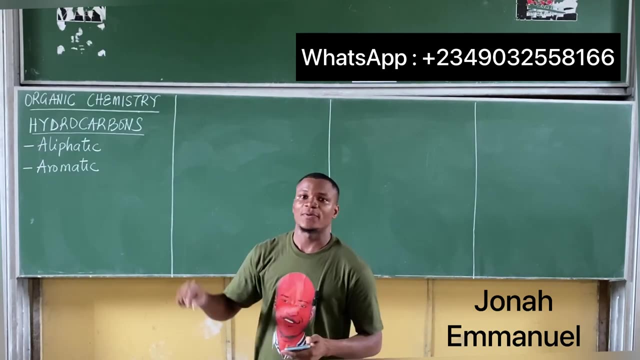 classes. On the bottom is aliphatic and aromatic hydrocarbons. Aliphatic and aromatic hydrocarbons: Give you one line space paragraph. One line space paragraph. Aliphatic hydrocarbons are open chain, not because they're oficarbons. 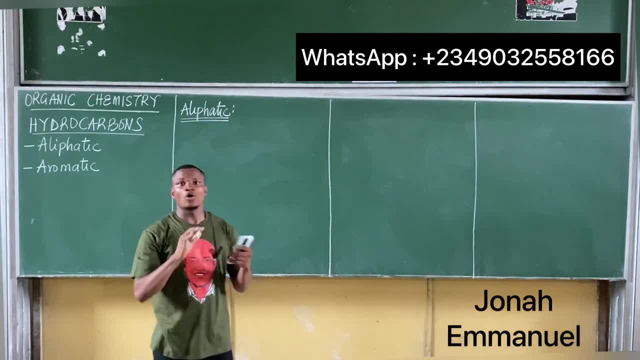 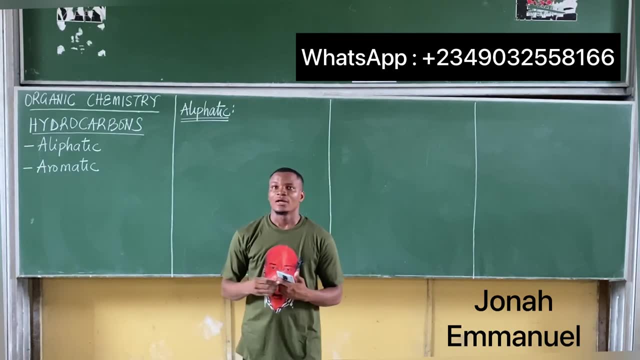 Aliphatic hydrocarbons are open chain. mamyµ vmusimuch eightication arké défamaya akирé Balência. hidrocarbons: Aliphatic hydrocarbons are open chain Compounds containing Aliphatic hydrocarbons are open chain compounds. 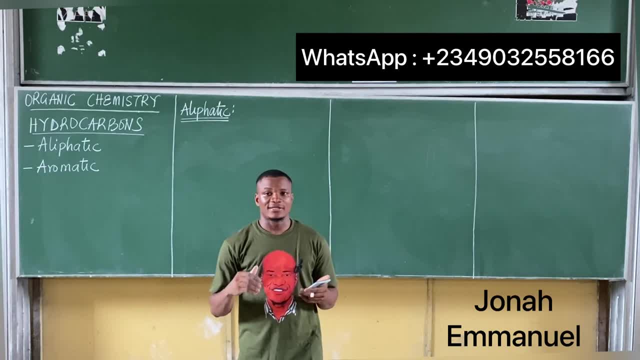 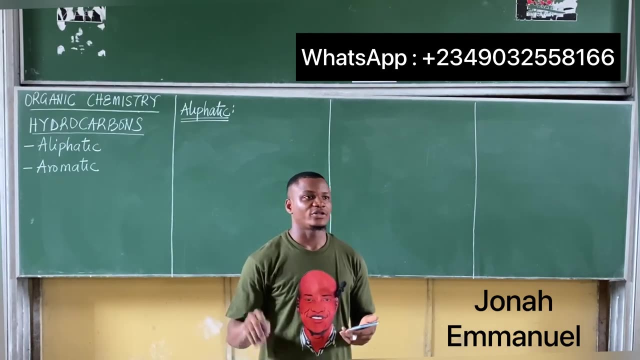 You can say Containing or that contains no rings. Containing or that contains No rings, R-I-N-G-S rings. that contains no rings. Who stopped? Whether they contain single, double or triple bond. Whether they contain single, double or triple bond. 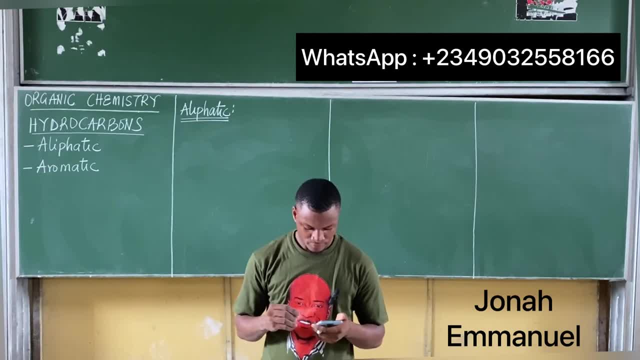 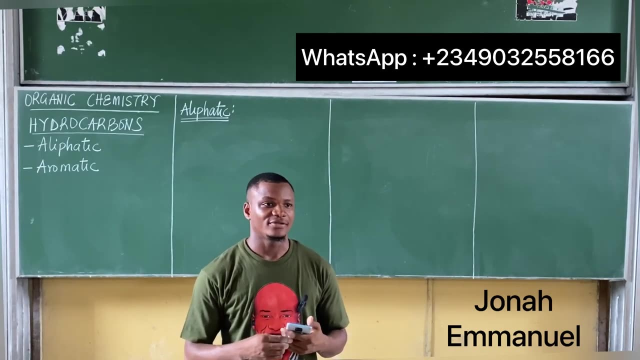 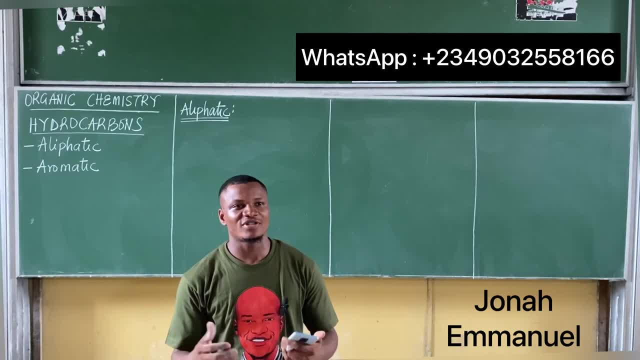 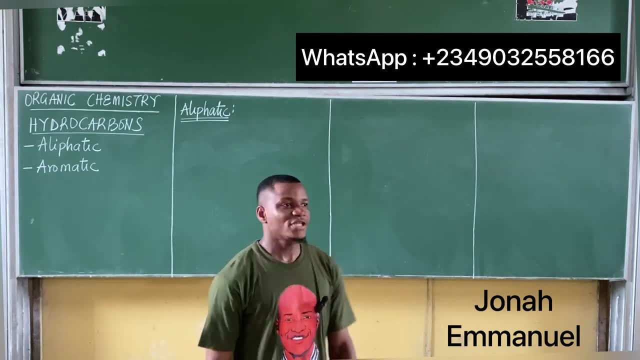 Alkenes are saturated. So if you want to use the word single bond, you say saturated compounds are compounds that contain single bond, in quotes only, Because even when you have a double bonded compound, eg something like this, Look at this, This is a. 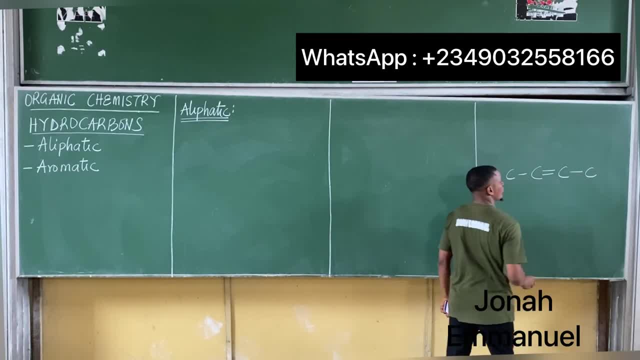 double bonded compound, Something like this: This is double bond, But observe, These two are connected by a single bond. That means, even in an alkene there's a single bond somewhere. So you don't just say single bond, because even alkene itself has. 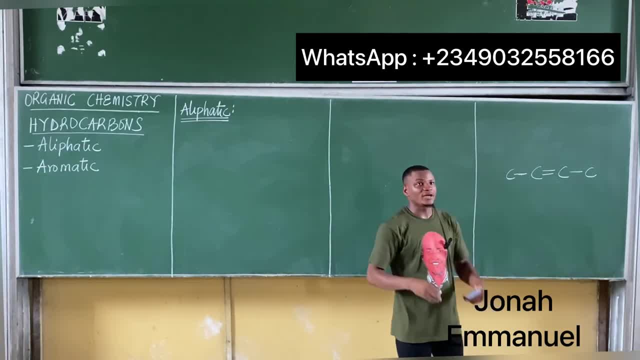 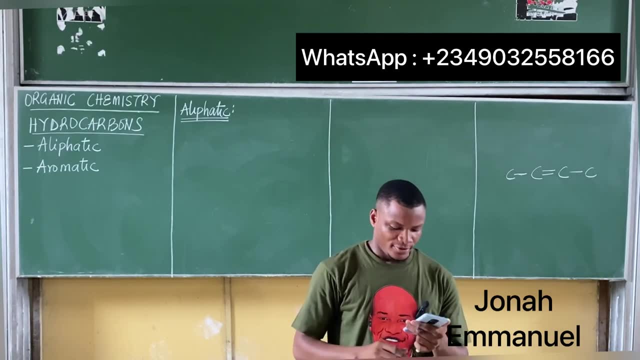 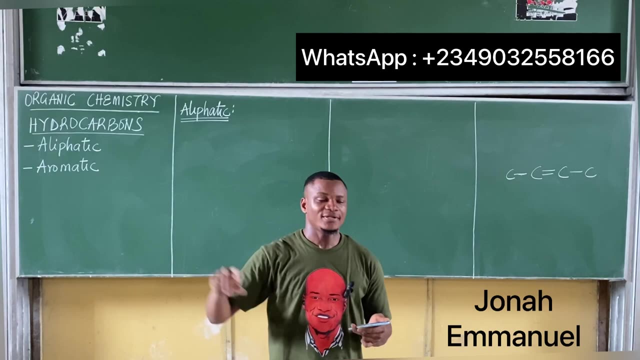 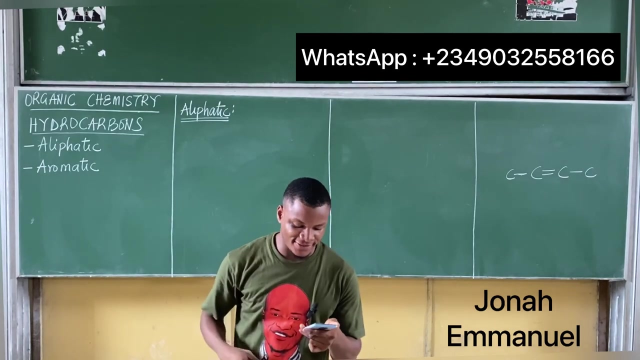 some parts where it is single bonded. So the idea would be: it is single bonded. only That's the key term there. Speak organic chemistry, Organic chemistry, Alright, First up, continue, please. Some aliphatics, Some aliphatics in brackets, like the cycloalkanes. 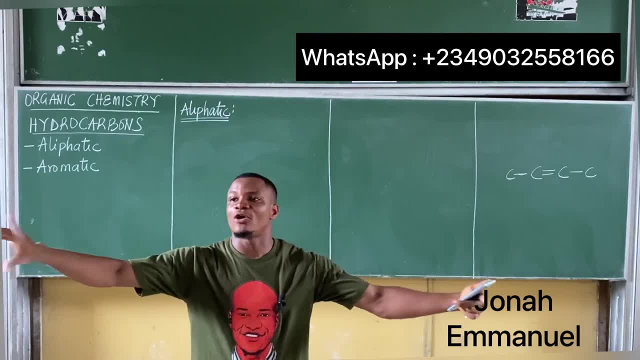 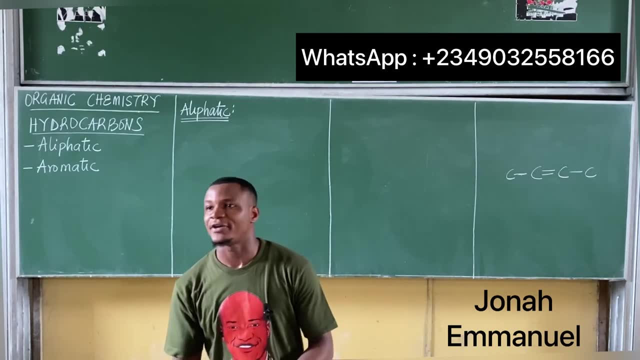 Some aliphatics. You said aliphatics are open chain compounds. Yes, Now, you are now adding something again. You are saying some aliphatics, like the cycloalkane. When I say cycloalkane, what does it mean? It means, it's what? there A ring. 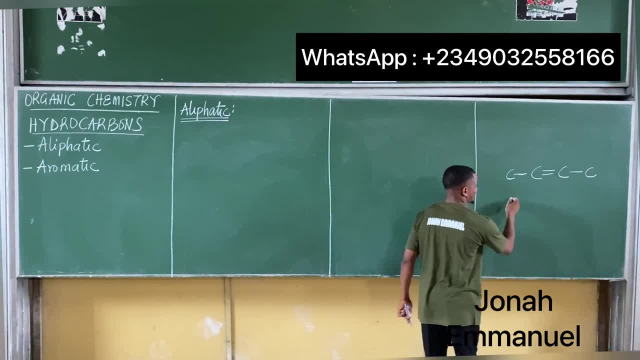 form And it's also what there: An alkane, A cycloalkane Example 1,, 2, 3.. This is single bonded. It's in ring form: Cycloalkane 1,, 2,, 3,, 4.. This is. 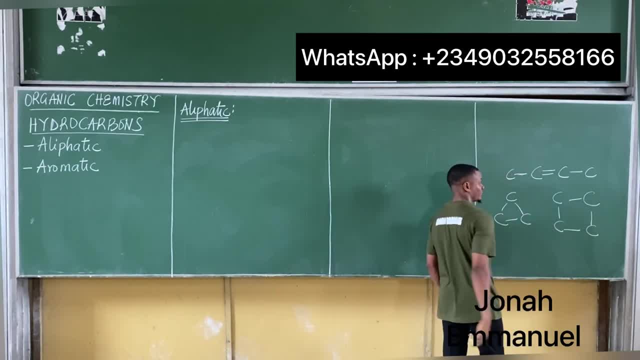 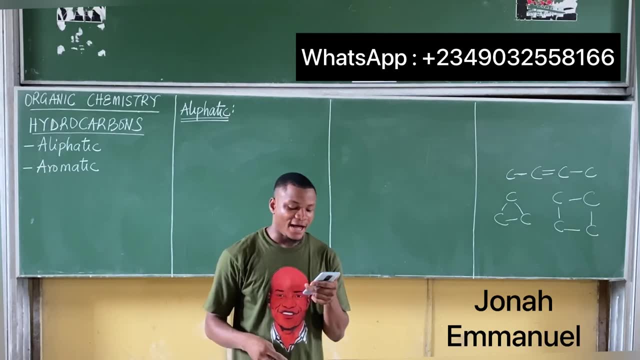 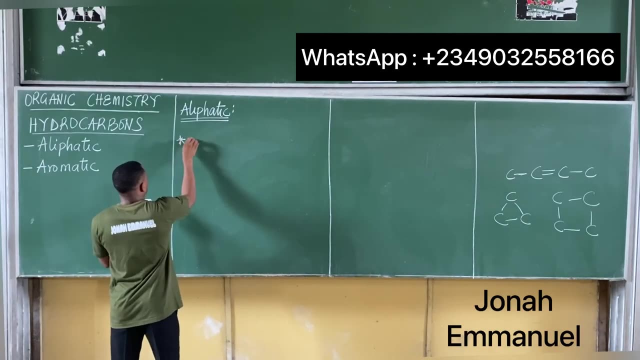 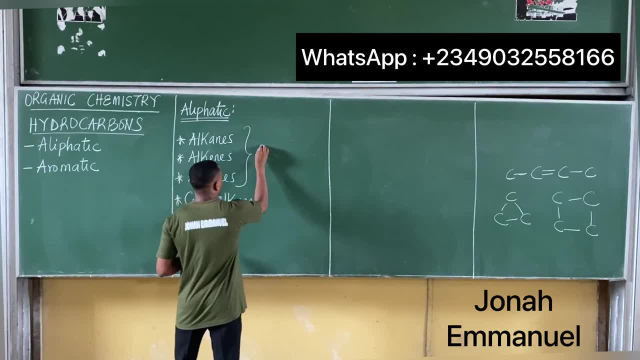 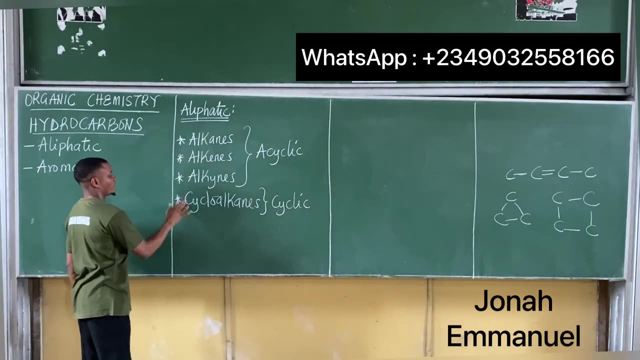 compounds. Alright, The aliphatics include 1,, 2,, 3, 4.. Alright, take another one. please Don't talk about aliphatic. Aliphatic include alkane, alkene, alkynes, cycloalkane. 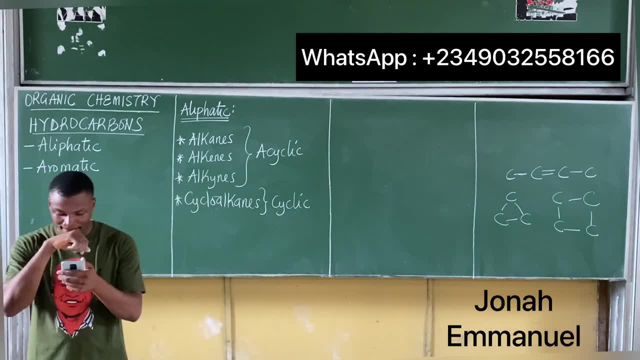 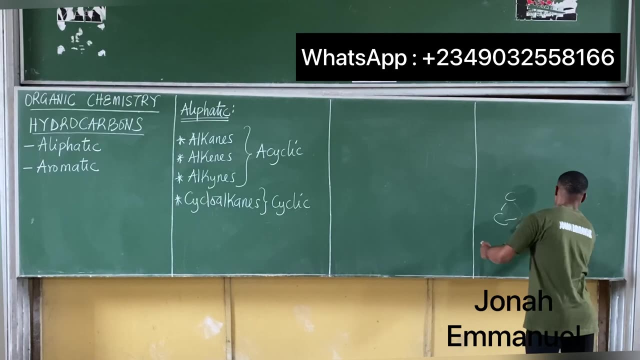 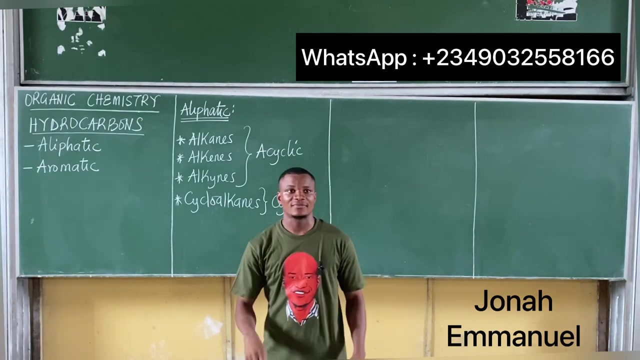 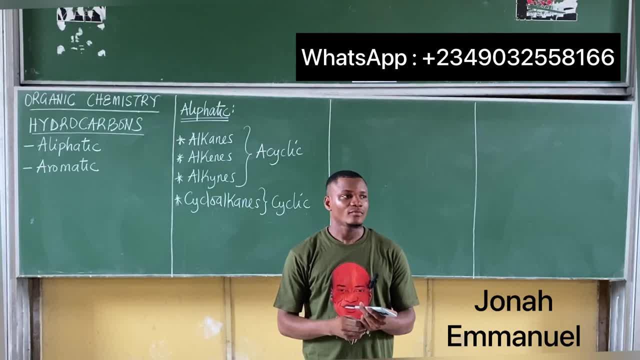 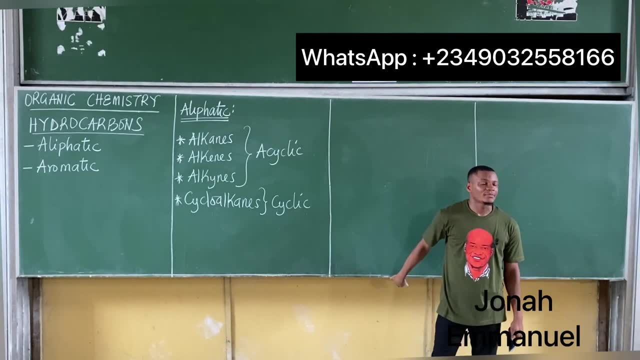 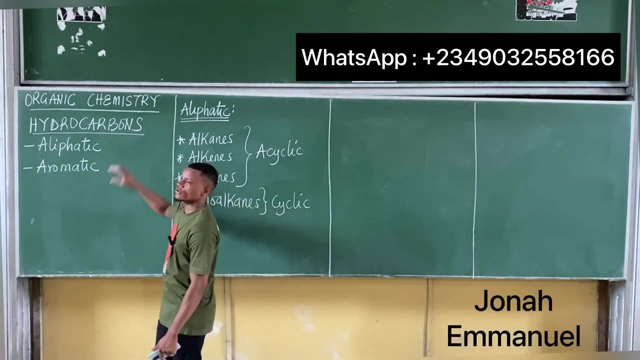 Cyclic, Cyclic. Alright, so look up, please, Look up, please. First things first, First things first, please. First things first. Now, this is weird, but that's how it is. We said: under hydrocarbons, based on their structure, we classify them as aliphatic and aromatic. 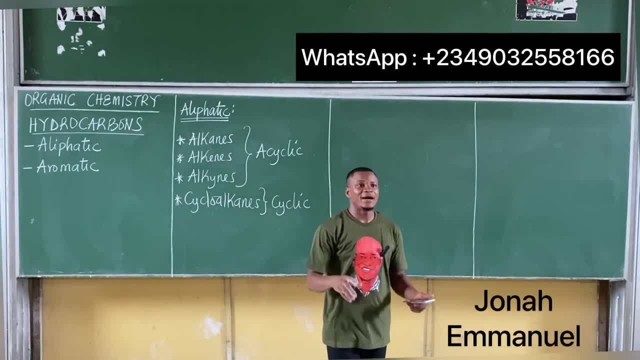 Now, what are aliphatic compounds? They are simply compounds that are not in ring form, In other words, they are open chain compounds. Example: the alkanes, the alkanes, the alkynes. But then what's weird now is this: I have things called cycloalkanes. Cycloalkanes are actually what they are: They are actually cyclic. That means they are actually ring compounds. 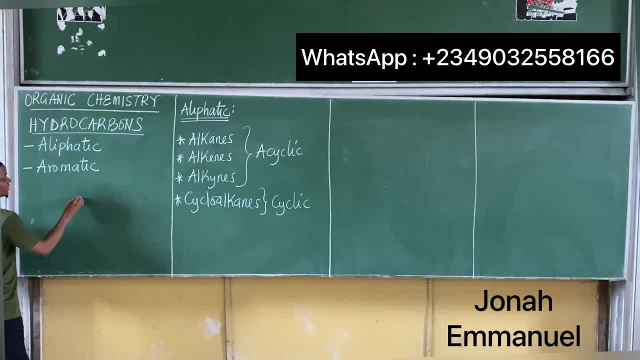 An alkane. a very simple example would be this: ethane, That's this one here. I will treat this shortly. We'll treat it shortly. So here's ethane. Observe that this is just a straight line like this. So we call this aliphatic, Why It's not forming a ring compound, It's just straight. So it's an aliphatic. 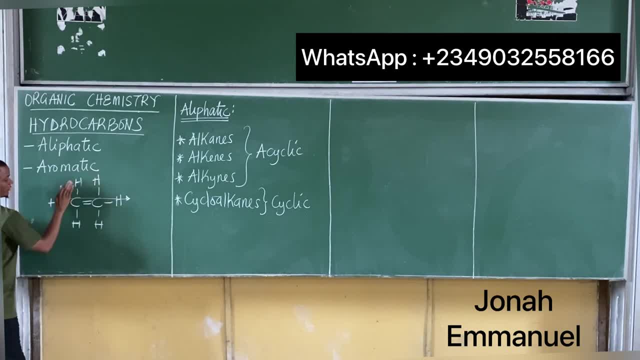 It was a double-bodied compound like this, So this one will go up. Something like this. This now becomes ethane Observe. it's still a straight line. I can choose to write how many carbons like this. It's still a straight line. 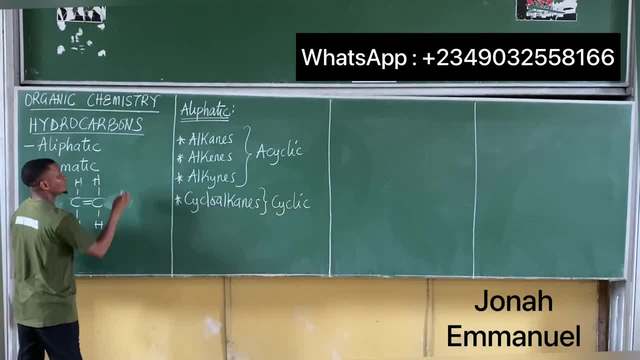 But then there's something weird For cycloalkanes: if it's a cyclo, that means it is forming a ring compound. Now, seeing this one here, the idea of cycloalkanes does not really perfectly suit the idea of. 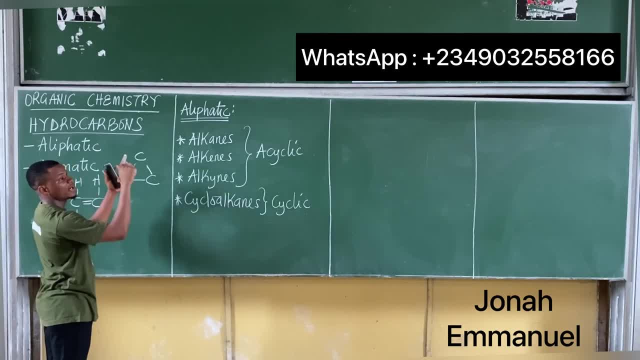 aliphatic, because we said aliphatics, they don't have a ring compound, But then note that there's an exception to that one there. So there's an aliphatic that has a ring-like structure and that's what there- the cycloalkane. So please take note of it. So there's actually an aliphatic. 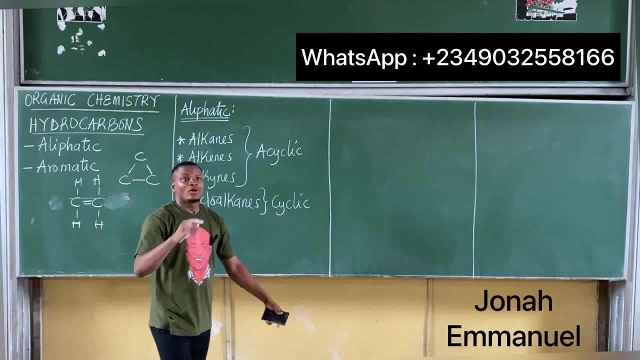 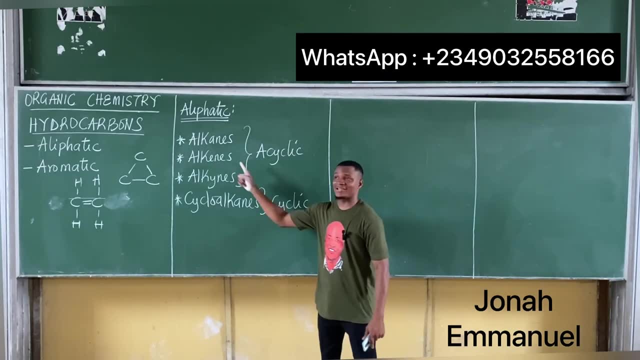 that is cyclic in nature. It's cycloalkane. What you should notice is this: Cycloalkanes are isomers of alkenes. You need this idea to do that past question. I'm just answering to you now. I think it's a past question. 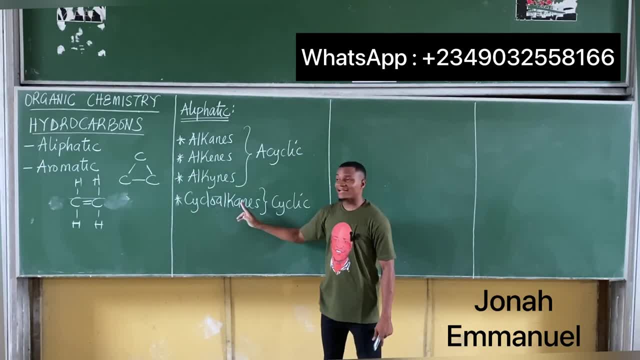 You need this idea to do that past question, So you can notice that cycloalkanes are isomers of alkenes. Please take note: Cycloalkanes are isomers of alkenes. Let me show you how that's done. I think the simplest cycloalkene I can get is cyclo-1,, 2,, 3, that's cyclo-propene. now let's take a propene, let's take the alkene equivalent. let's take propene for a propene. 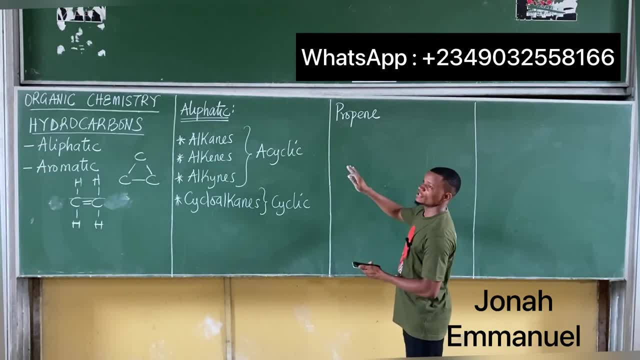 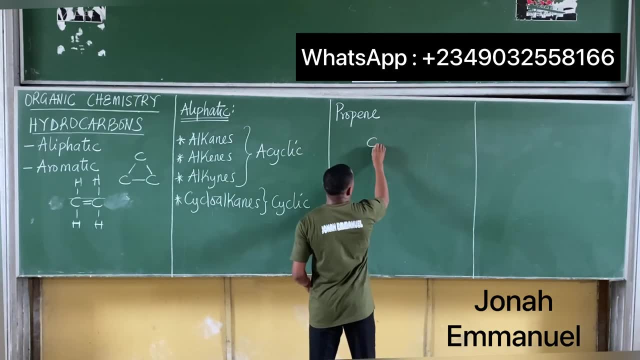 is not a proper name. it should be one propene, but let's assume for now it's propene. we'll discuss this one much more later. so let's look at propene. for propene, I expect three carbon atoms, so 1,, 2, 3,. for an in I expect a double bond, so perhaps double bond your. 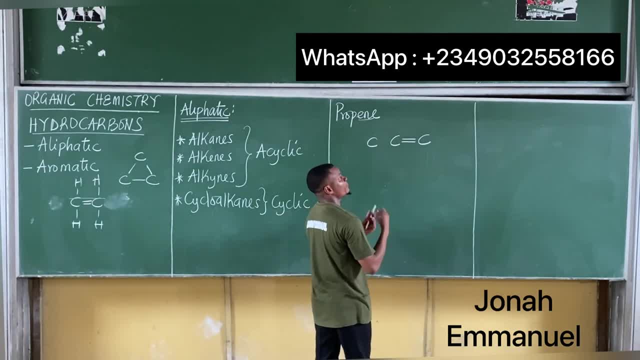 next steps now will be fill this up. we said for a proper balanced carbon atom each of them should have four bonding. so this one has 1, 2, 2 is left. I have 3 and 4, this: 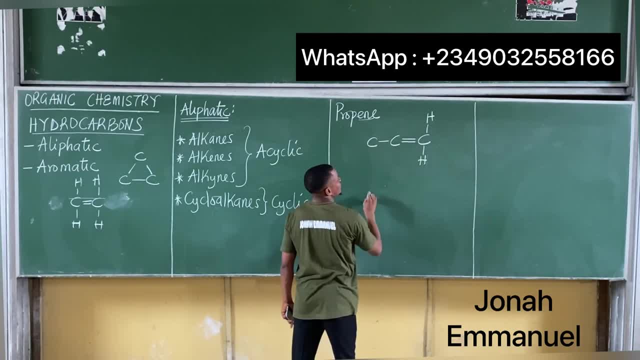 one has 1, 2, of course these two will be connected by this. so this one now has 1, 2, 3, 1 more. Next is 4,. this one has 1, 3 is left 2, 3 and 4, so from this one here, this is an. 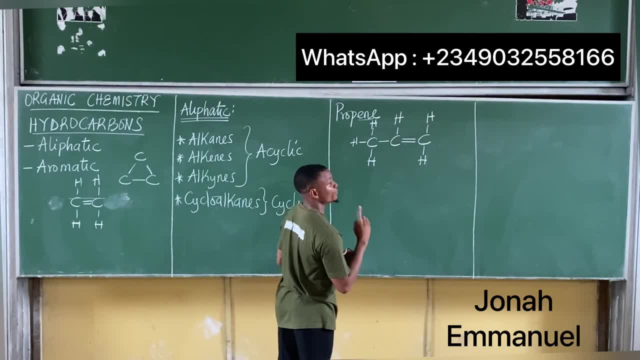 alkene, that's propene, or better still, one propene. I'll tell you why it's one much more later. If I want to get the molecular formula of this, I'm having three carbons: 1,, 2, 3, so 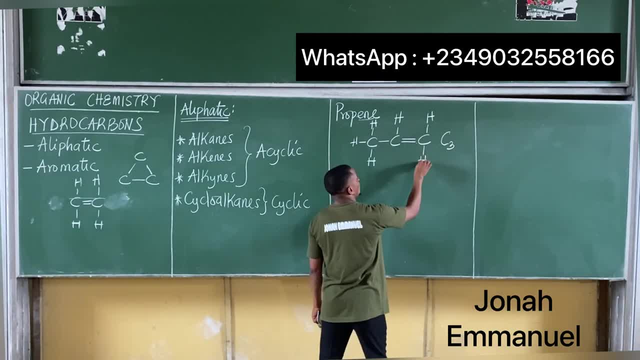 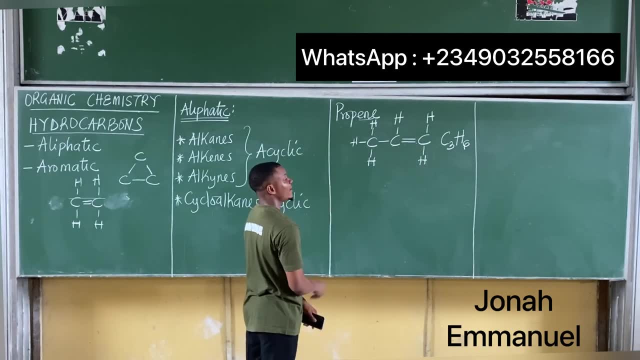 it becomes C3,. I'm having how many hydrogen there: 1,, 2,, 3,, 4,, 5, 6, H6, so propene is C3H6.. Let me get the cyclocarbons. 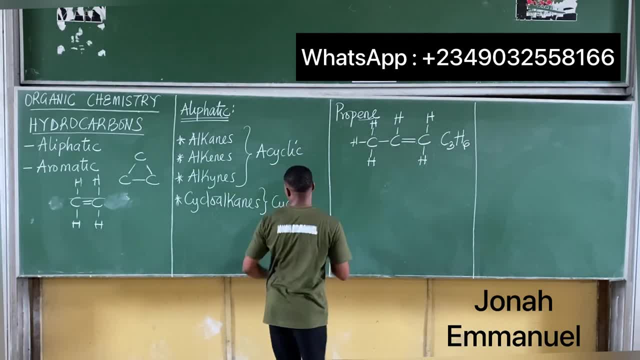 This is the single counterpart of this in its alkene formula. now we said cyclo and alkene. it is an alkene, that means it's a single bond. so let's have three carbons forming a ring-like structure and all being connected by a single bond. single bond here, single. 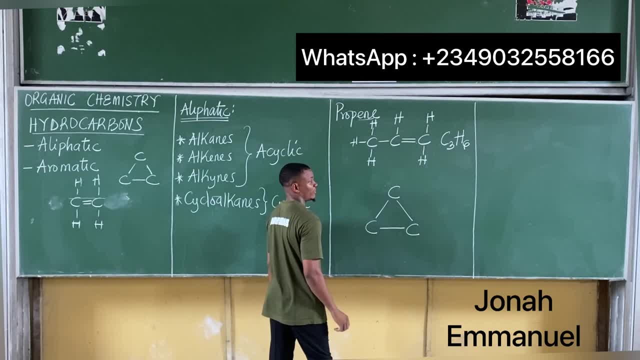 bond here, single bond here. My next task will be to balance them up. this one has 1,, 2, 2 more left, so H2 to make it 4.. This one has 1,, 2, 2 more left. I have H2 to make it 4.. 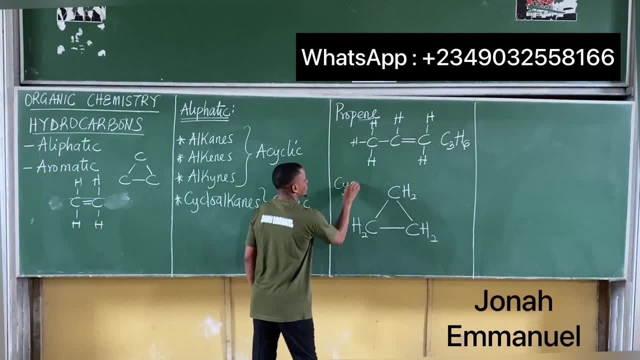 If I want to get the molecular formula of this, it becomes a cyclo- cyclo. I'll tell you why it's cyclo in the last class, because it's a ring-like structure. then a propene- propene because I have 1,, 2,, 3, 3 carbons, and then it's an alkene single bond. it becomes: cyclopropane. This one becomes 1,, 2,, 3, C3H2,. 2,, 2,, 3,, 4,, 5,, 6,, 7,, 8,, 9,, 10,, 11,, 12,, 12,, 13,, 13,, 14,, 14,, 15,, 15,. 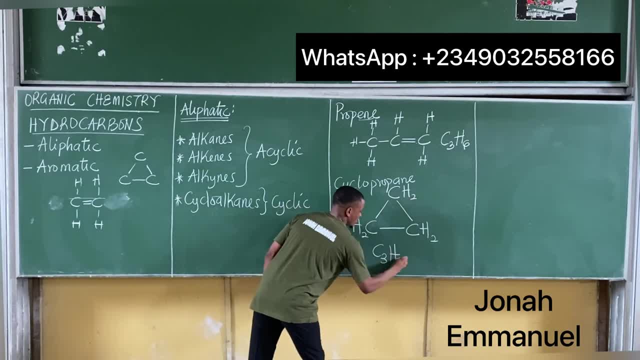 16,, 16,, 17,, 18,, 19,, 20,, 21,, 22,, 23.. C3H into 2226.. Observe that both of them have the same molecular formula but different structures. So I'm saying that prop-alkenes and cyclo, not cyclo-alkene, sorry, not cyclo-alkene. 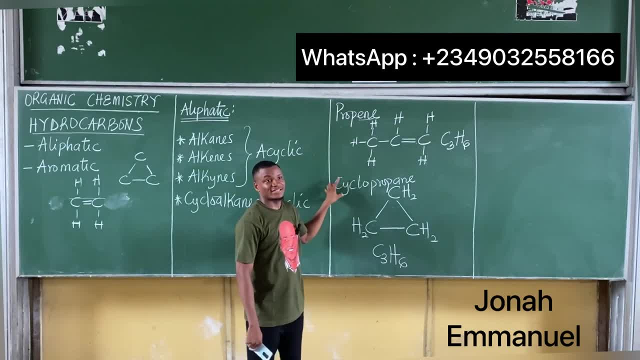 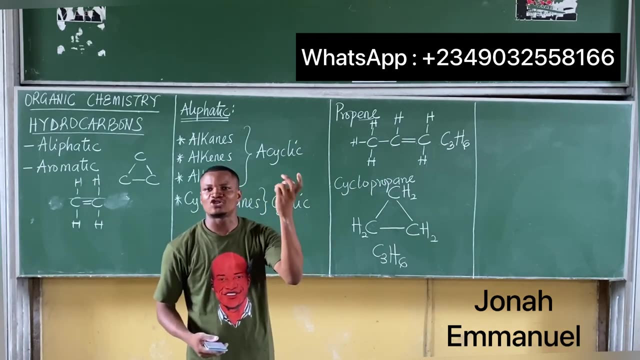 but cyclo-alkenes, alkene and cyclo-alkene are isomers. Please take note, They're isomers. They're isomers. I see you. What kind of isomers are they? Chain isomer, functional isomer or geometric? 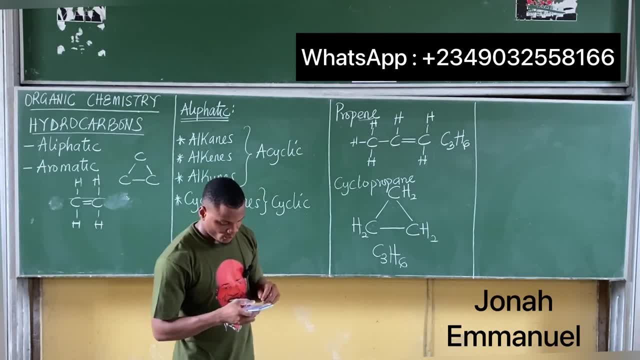 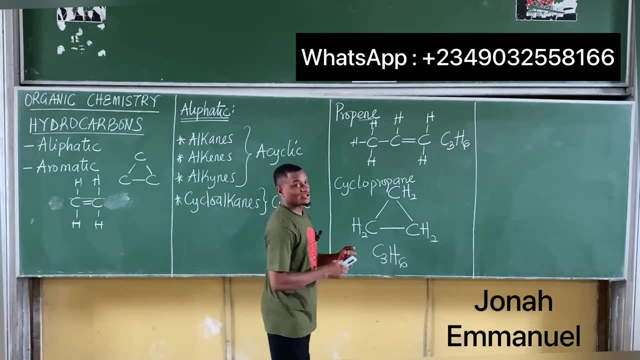 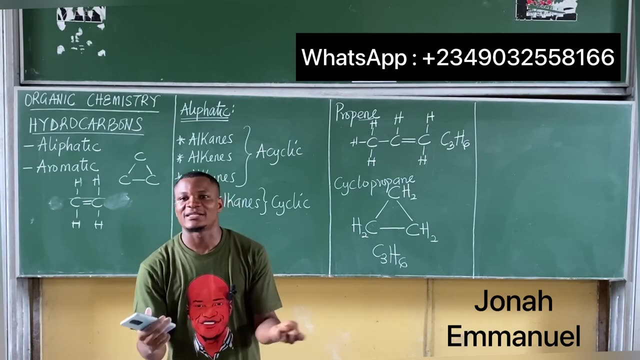 Huh, What kind of isomers are they? Is it chain isomers? We did three types of isomers in the last class. We did chain, we did functional, we did geometric. So when we say they are isomers, what type of isomers are they? Huh? 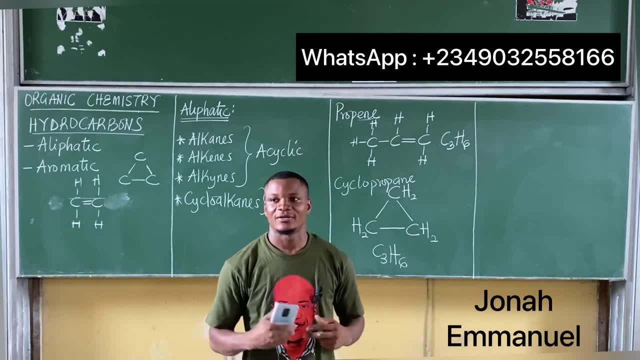 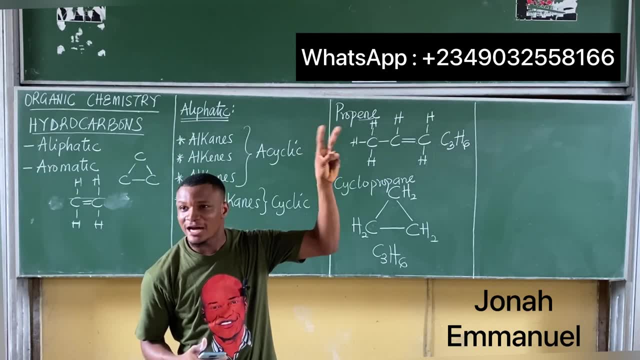 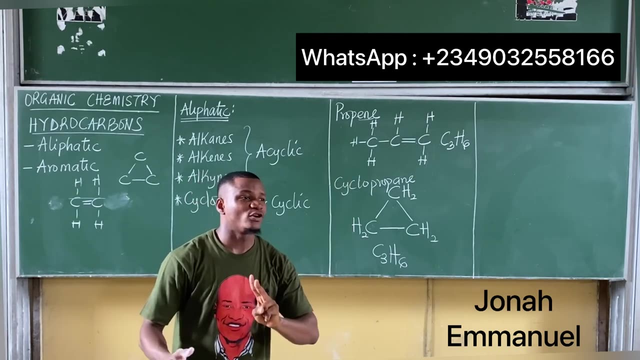 What is a chain isomer For chain isomers? what happened there? They have what there? The same molecular formula. What again there? The same functional group, Is it not? Check your notes? Same molecular formula, same functional group, but what there? Different arrangement of what Atoms in space. 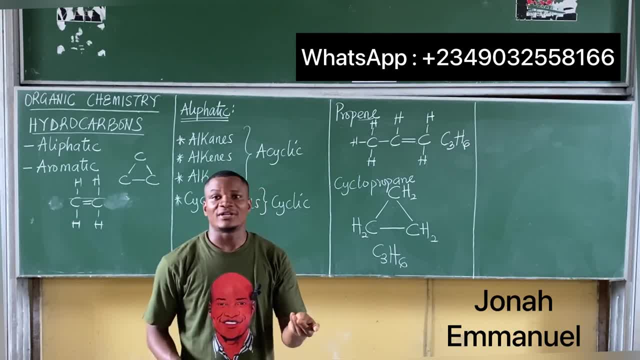 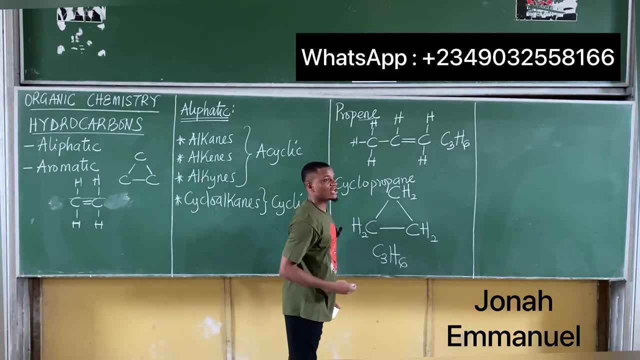 What is a functional isomer? They have what there? The same molecular formula, but what there? Different functional group. Look at this one here. These two have the same molecular formula, C3H6, C3H6. But they have different functional group. 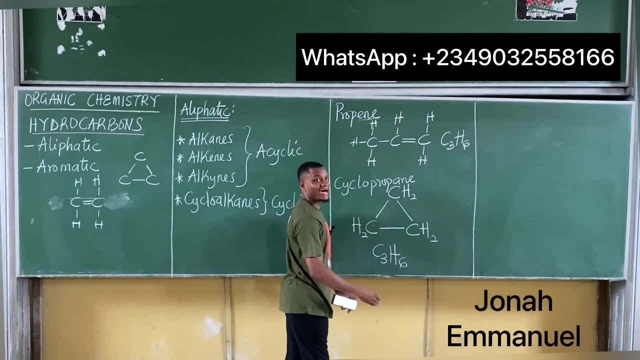 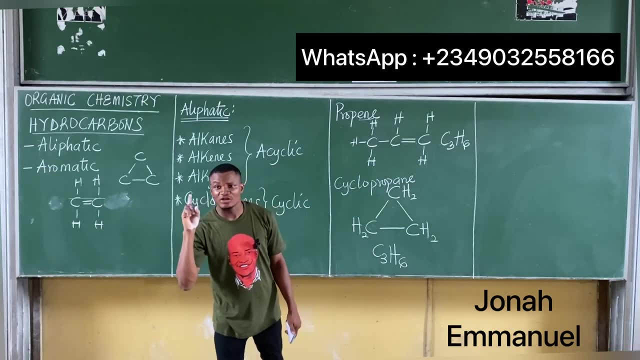 For this one here the functional group is what there A double bond That becomes what there An alkene. For this one here it becomes what there, A single bond That becomes what there An alkene. So it's what there, A functional isomer, not a chain isomer, Please. 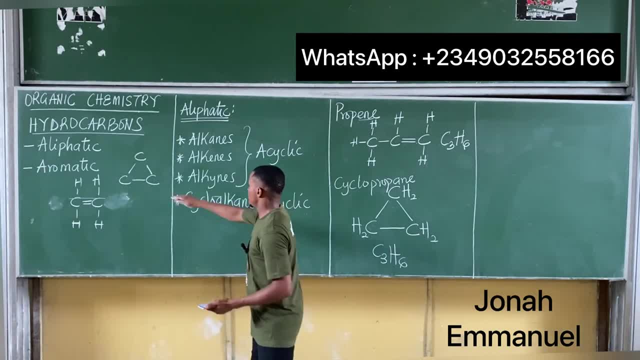 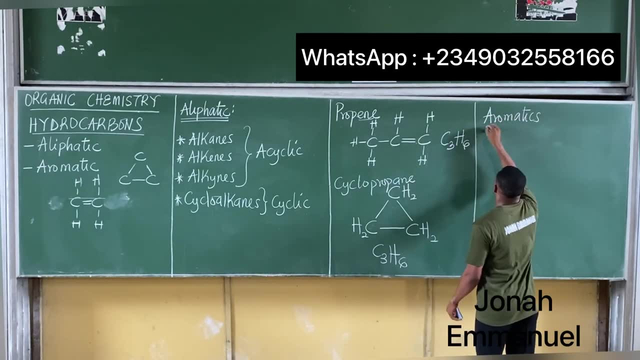 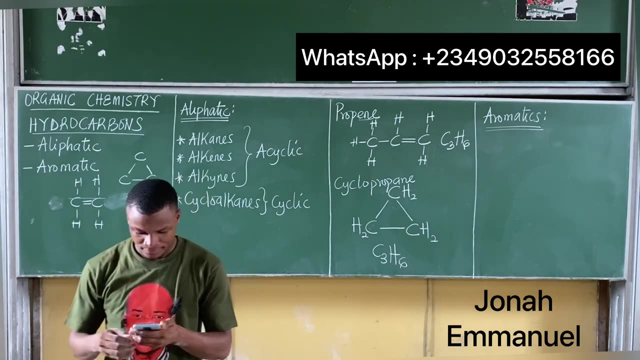 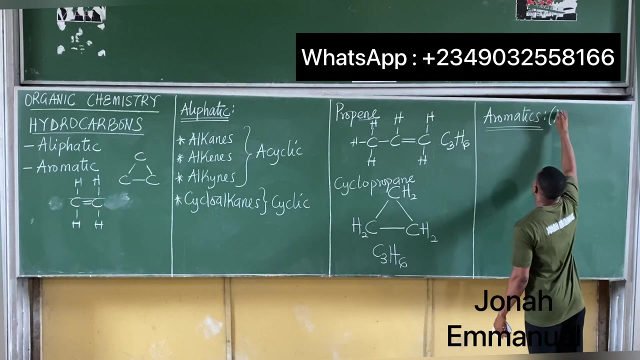 Alright, let's proceed. Let's now look at aromatics. before we move on, please, Let's now look at aromatics. Let's now look at aromatics: Aromatic hydrocarbons- aromatic hydrocarbons, also called arenes. 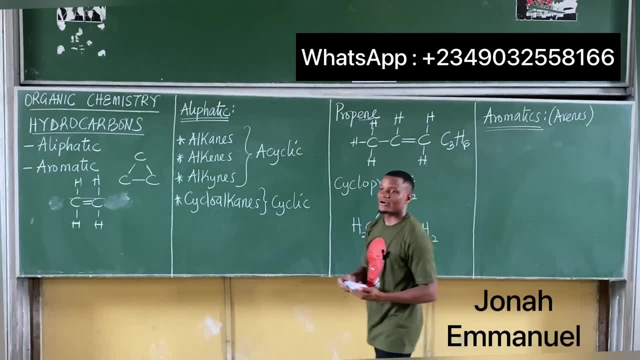 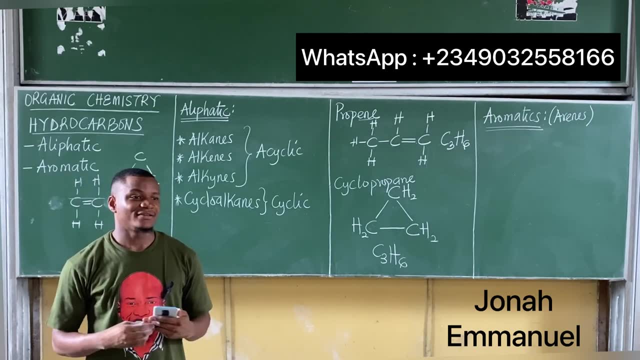 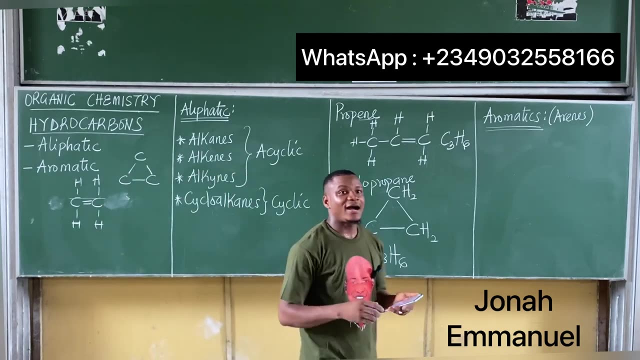 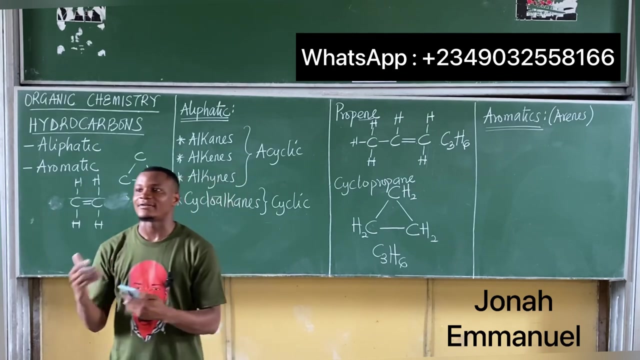 Aromatic hydrocarbons, also called arenes. there it will come to pass. I said arins, not arinze. I said arins also called arins acyclic, aromatic, acyclic. so you call them either the aromatic or the arins. 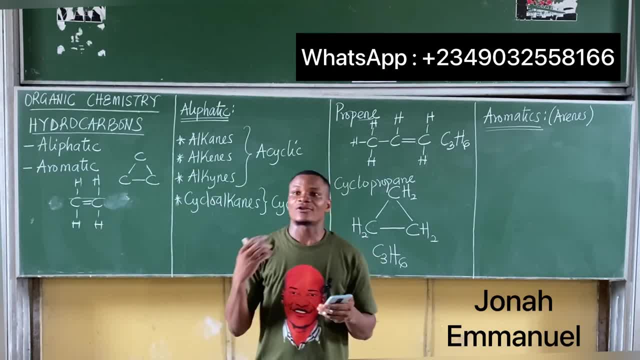 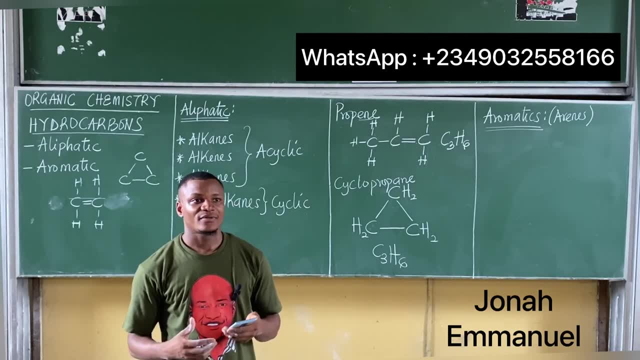 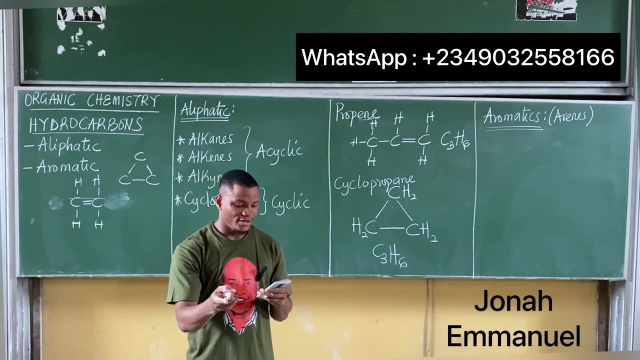 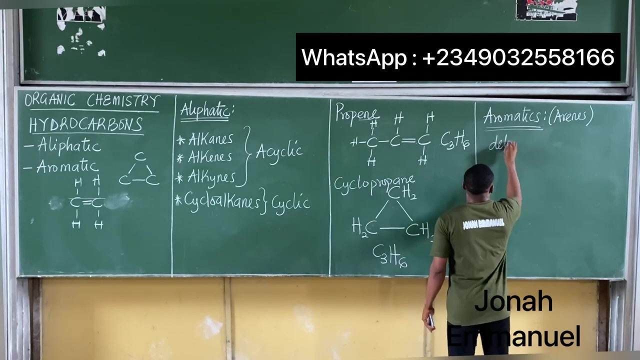 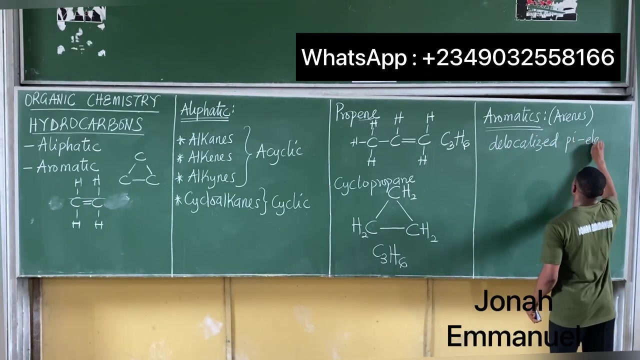 acyclic that consists of conjugated planar ring systems. that consists of conjugated planar ring systems accompanied by delocalized- accompanied by, this way, delocalized pi electron. I'll explain what this means one more time. one more time we start doing the arins. I'll tell you what a delocalized. 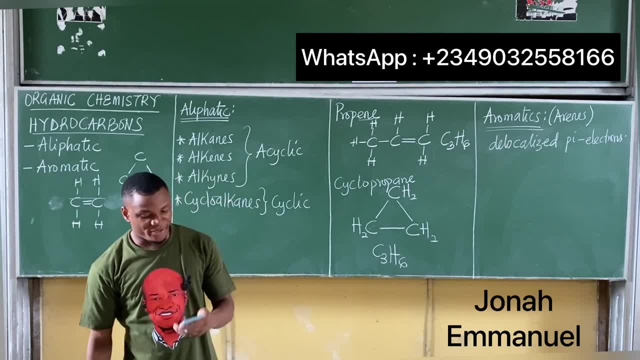 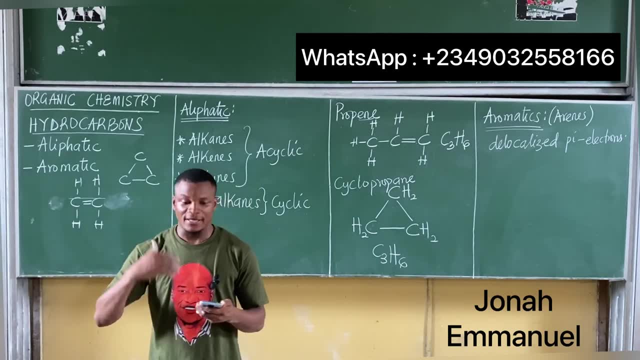 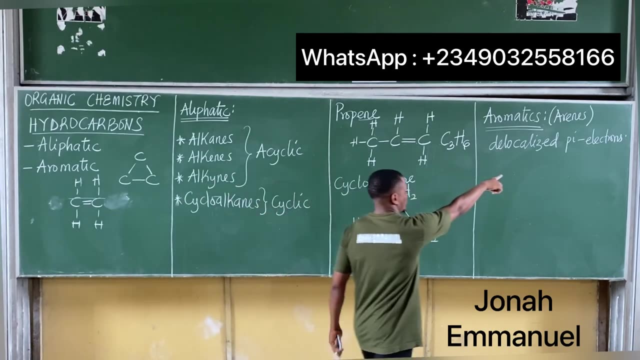 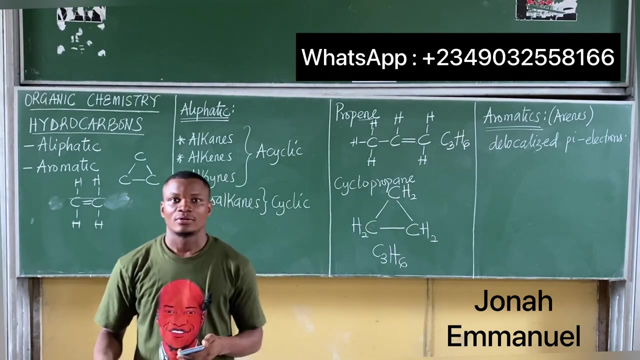 pi electron means how we start treating arins accompanied by delocalized pi electron cloud. delocalized pi electron cloud. electron cloud pi electron- this one here- pi electron cloud cloud, c-l-o-u-d cloud of the house. let's use electron, then clouds. 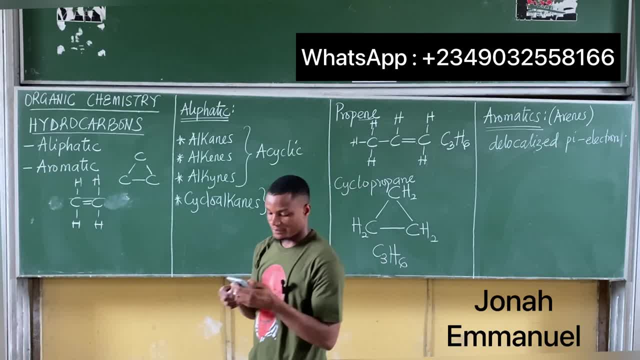 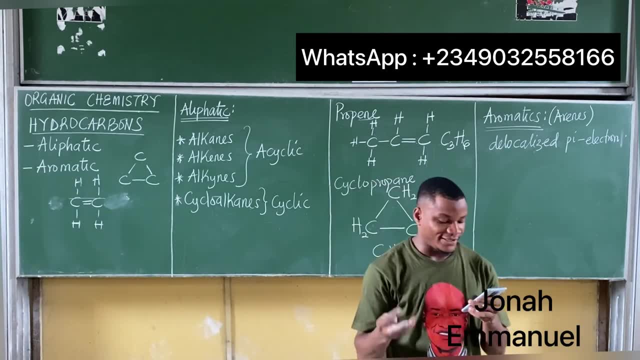 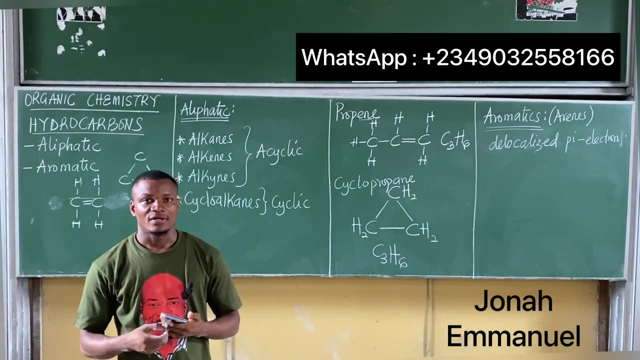 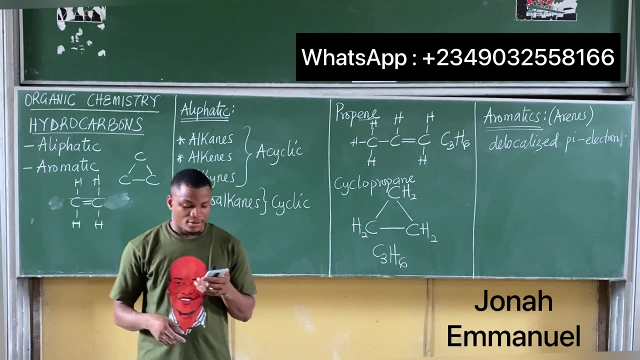 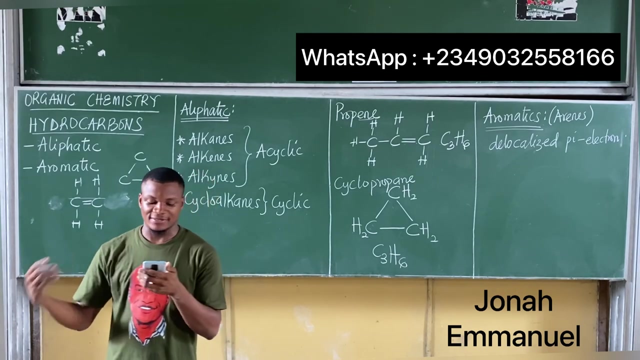 electron then clouds. plural form in place of individual. in place of individual. alternating, double and single bonds in place of individual, double and single bonds in place of individual alternating, double and single bonds accompanied by the localized pi electron clouds in place of individual, alternating, double and single bonds.